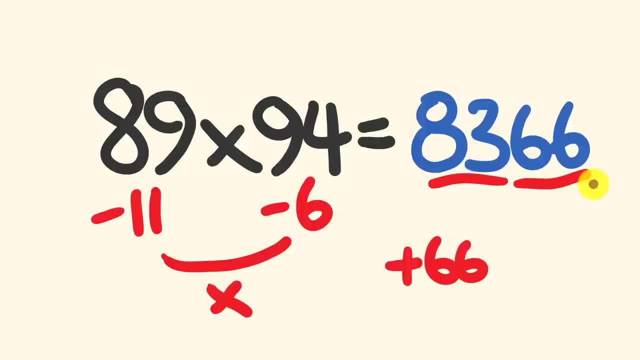 How's that? As easy as promised, right, And your homework here is to see why this works, And I'm going to pin the best answers in the comments. So what about a few for you? Remember, the very first thing we do is we're going to work out the distance from 100.. 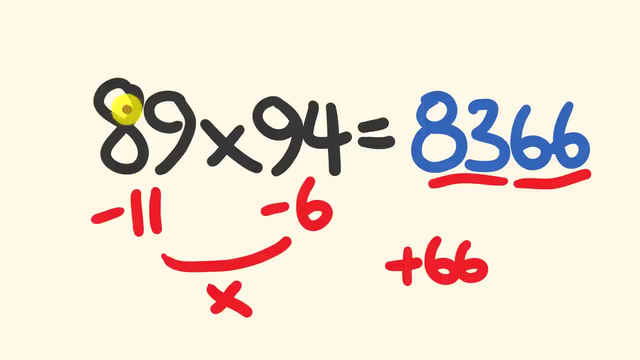 Then we're going to put one of the numbers we're multiplying with one of the differences there And that will give us the first part of our answer. Then we multiply these two. We're going to put the two differences here to get the second part of our answer. 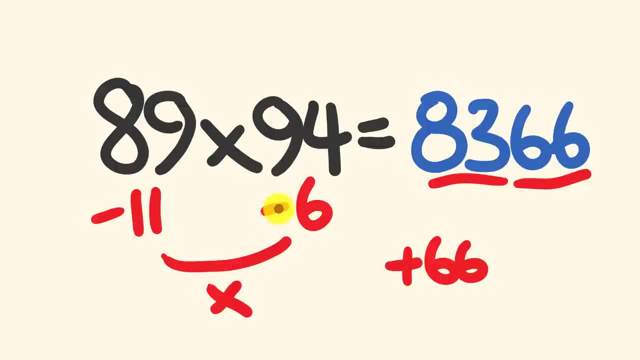 Just watch out. If this number is over 100, this will be a positive number, And when we multiply it'll give us a negative here. So just watch out, That will occur in the third example. Just be careful with that one, and I'll go through how to solve these sorts of questions when I show you the working out for that one. 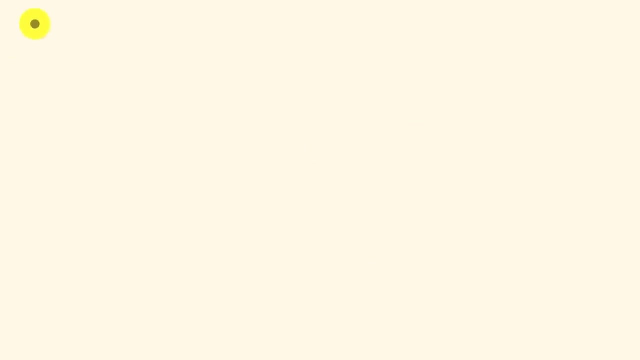 So what about a few of these that you can do? Okay, so first off, we have 95 multiplied by 93.. I think you should be able to do that one, no problems. What about we go over 100? now? We'll go 109 multiplied by 102.. 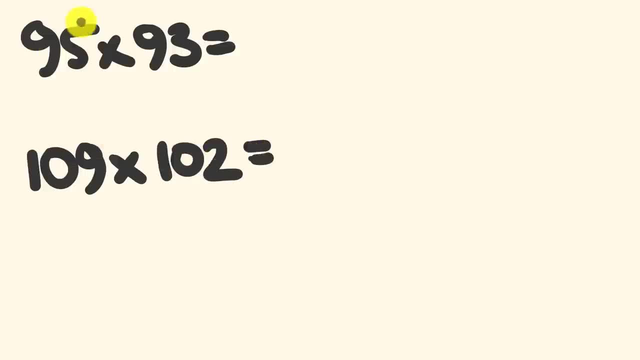 Obviously, those differences are now going to be positive differences as opposed to these which were negative differences. They're under 100.. These are over, And then we're going to do one above 100 and one below 100. What about? we do 88,, which is below 100, multiplied by 104. 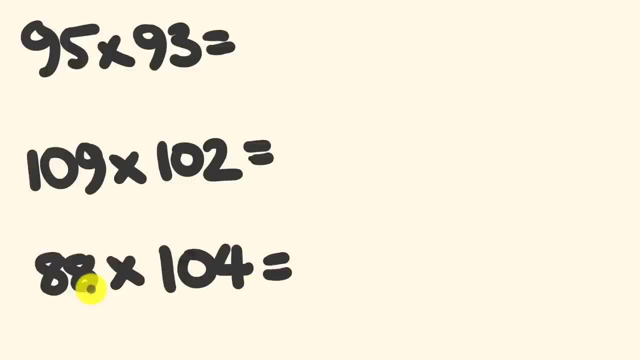 And, as I said, just watch out That final step. you're going to end up subtracting that part of your answer. You'll see when I go through the working out here. So pause the video, hit the like button, give these a go and leave something lovely in the comments for me to read, or at least something funny. 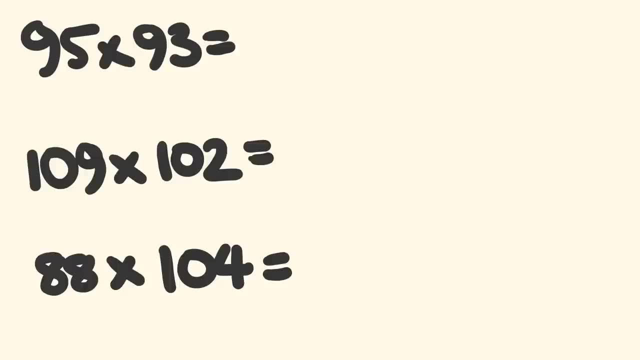 And then we'll see how you went. Okay, you done that. I'll be checking. So let's have a look at the answers here. So, first off, 95 multiplied by 93. You can see that from 100, this is minus 5 and minus 7.. 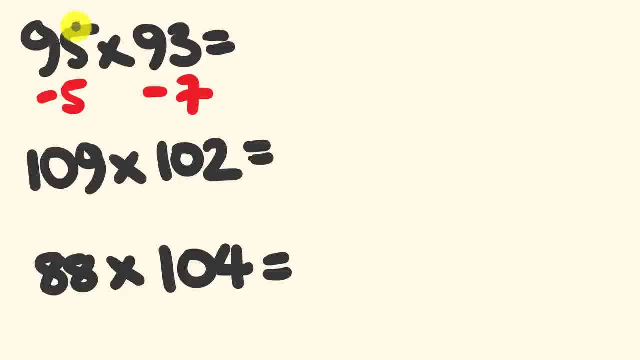 Okay, what do we do now? Well, we're going to go 95 minus 7,, which is going to give us 88.. Nice and easy, And that's the first part of our answer: 8,800.. And then negative 5 multiplied by negative 7 gives us an answer of positive 35.. 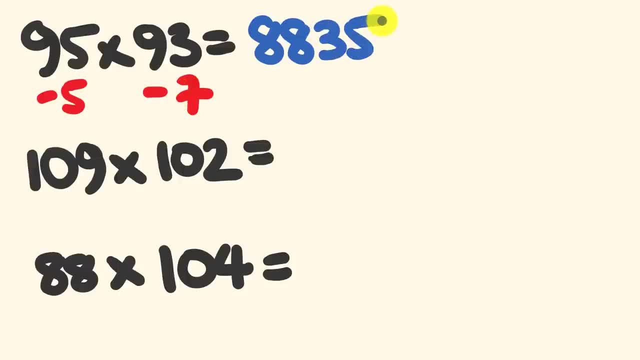 So we're just going to put 35 on the end there, Our answer: 8,835.. How'd you go with that one? Okay, the next one: 109 multiplied by 102.. How far from 100?? Well, this is now above 100. 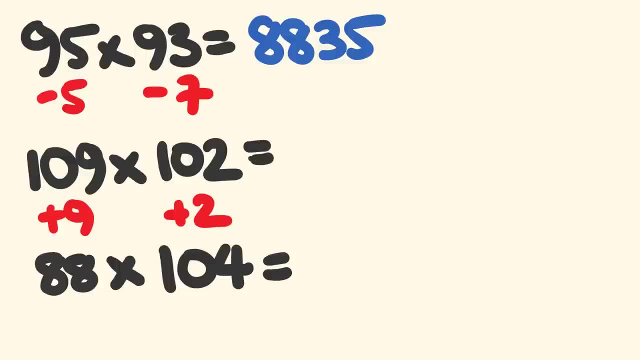 This is positive 9, and this one here is positive 2.. So when we put these together, we're going to go 109 plus 2,, which is going to give us 111,, the same as 102 plus 9.. 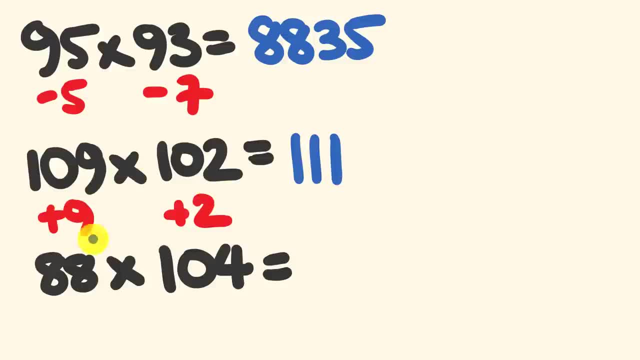 Gives us 111.. The next step: we multiply these as we did before: Positive 9 multiplied by positive 2, well, that's a positive 18.. So we're just going to add 18 to our answer. Our answer: 11,118.. 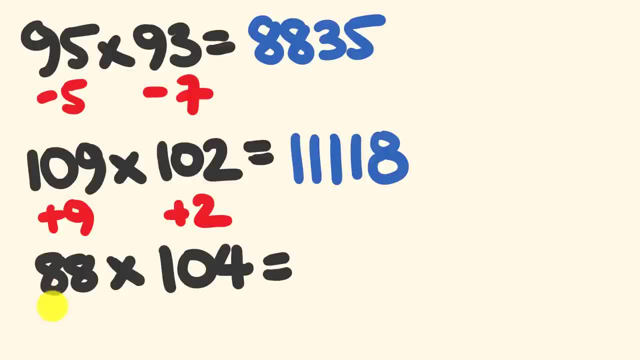 So to the final question: 88 multiplied by 104.. How far is each of these numbers from 100?? Well, 88 is 12 under and 104 is 4 above. So we have negative 12 and positive 4 as our differences. 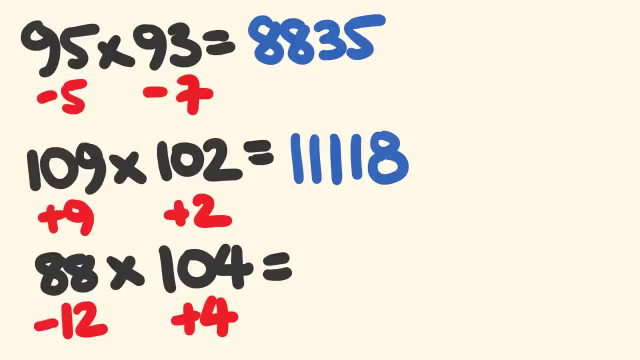 So 88 plus 4, the answer to that is 92. And you're going to see, this is exactly the same as 104 take 12, also 92. The difference now comes in this part. here, As you can see, negative 12 multiplied by positive 4,. 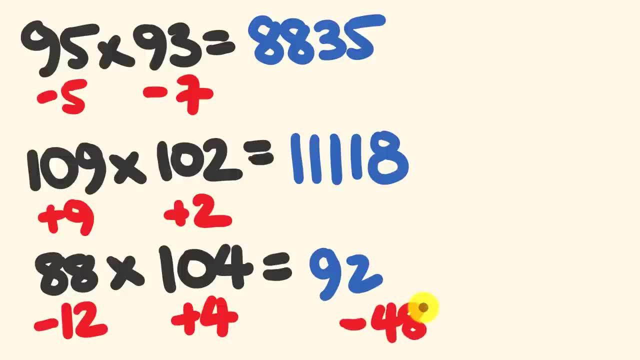 this gives us an answer of negative 48.. So instead of adding this to the end, like we did before, we're going to actually take this from this number here, which is actually 9,200.. So what do we get when we do that? 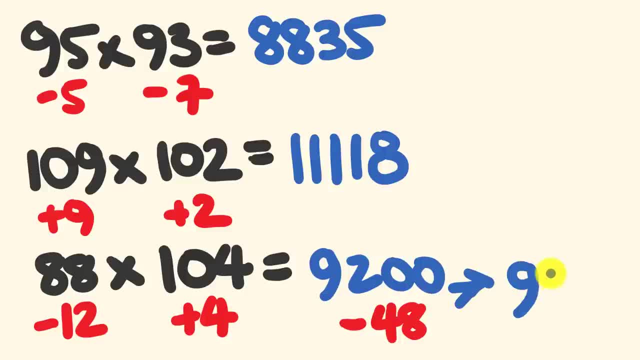 Well, no problem, We're going to get the answer: 9,152.. I hope you got that one. Anyway, it's a cool trick, right. Once again, big call to action Like subscribe, interact. The algorithm commands you. 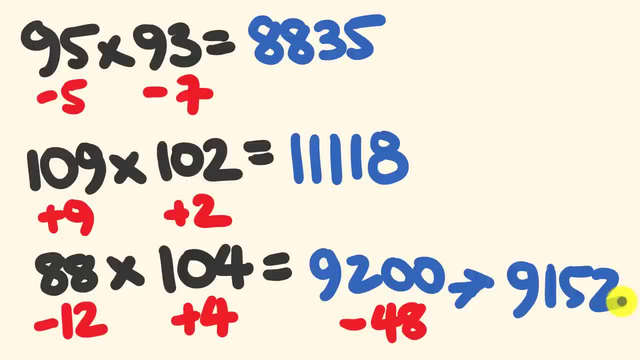 And, as usual, a big thank you to my Patreon. There is a link in the description below if you wish to support my channel. Anyway, we'll see you next time. Bye.